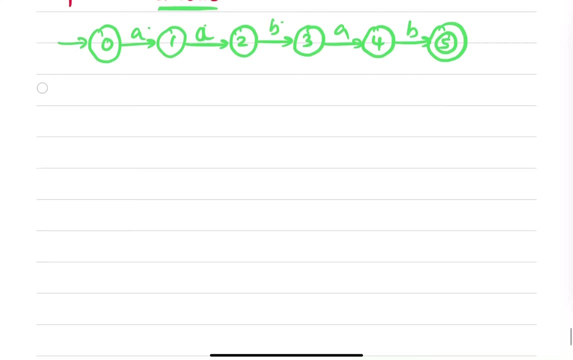 see more examples of transit table in the videos. So what are the inputs? We have just two inputs, A and B, and states are 0,, 1,, 2,, 3,, 4 and 5.. So the basic entries: on 0, you are going to 1 by taking input as A. So on 0, taking input A, you are. 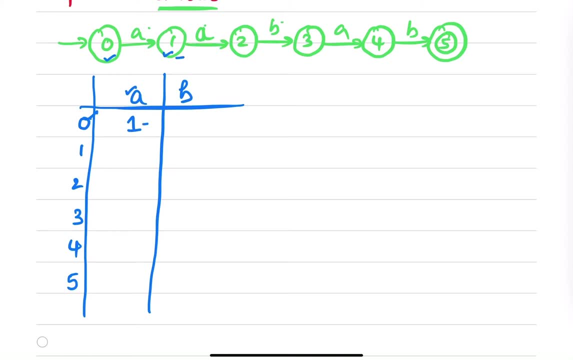 reaching to 1.. From 1 you are going to 2 on taking input a, and from 2 you are reaching to 3 on taking input b. from 3 you are reaching to 4 on taking input a, and from 4 you are reaching to 5 on input b. 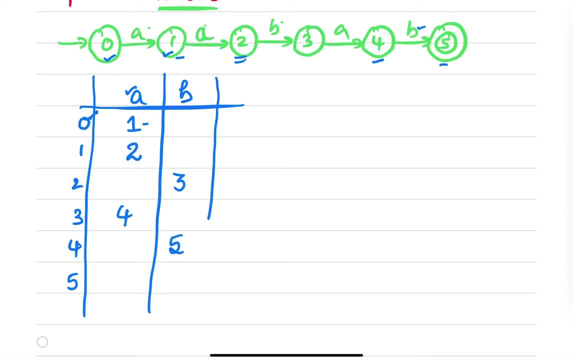 and for fifth, we can't say anything right now, let's find out the prefix table values for the given function. so here, at zero state, you have, you don't have anything, so it will be zero at one. you have a, so you will write a, and you have to fill position for b, so you will add b to. 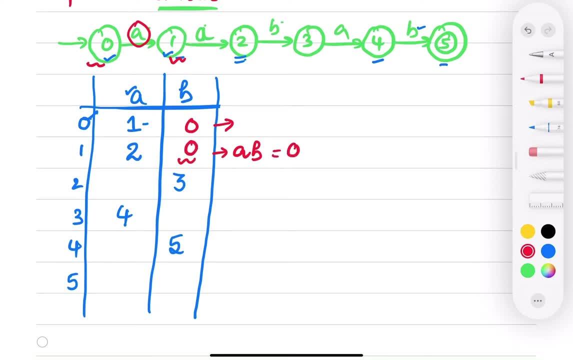 it and you will find the prefix value, which is zero, right. a doesn't matches with b, correct. to know how to find the prefix value, you can check previous videos. now here at state 2, you have a right and you have to fill this a. so if you check the prefix value for, 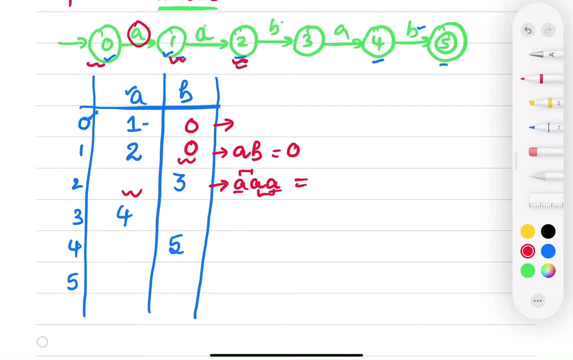 this, you will get a 0. and if you check the prefix value for this, you will get a 0. and if you check this, a matches with a and a matches with a right, so it's 2 correct. then for three, if you have reach to here and let me change the color, and here you have a, a b, right. you are here right. so a, a b. 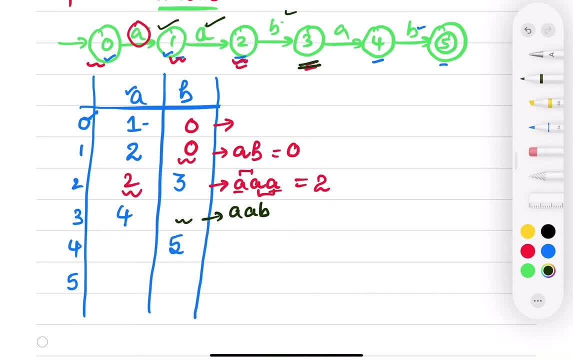 has been covered and you need to fill this position. that is d. so if you check the value, a matches with b and a? a doesn't matches with b? b and a, a, b doesn't matches with b? b, so it's zero right. and for fourth one, if you check, you are here, you have reached a, a, b, a and you have to. 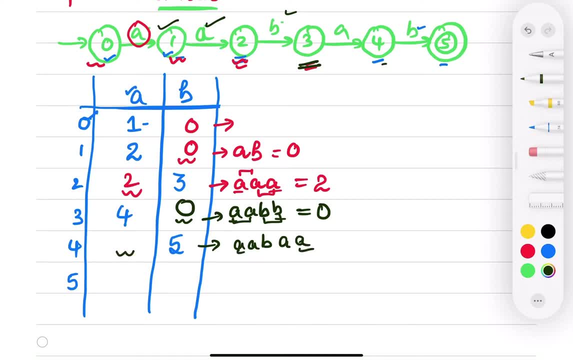 fill this position. that is a, so a matches with a, a, a. matches with a, a, a a b doesn't matches with b a, a, a, a, b, a doesn't matches with this. so two: right now, here you don't have anything and you have reached here. so a a, b a, b, a, a, b a, b. am i right? and you have to take for this and this. 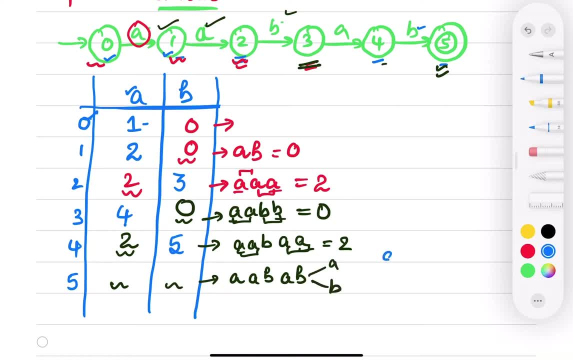 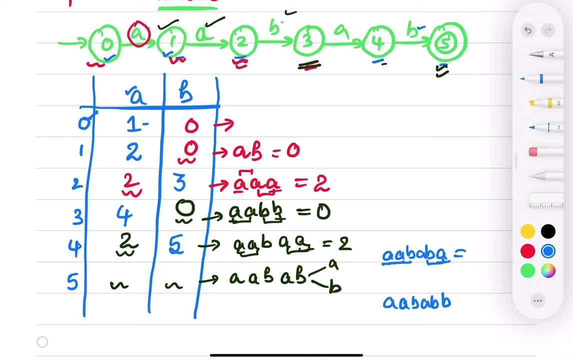 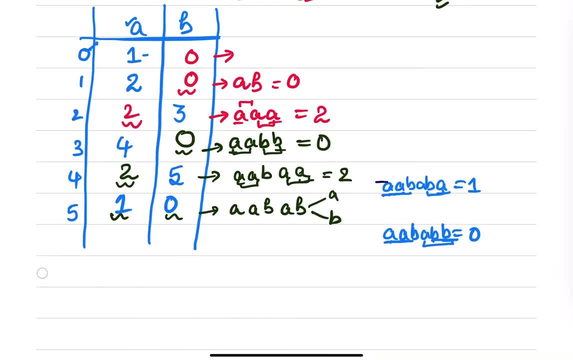 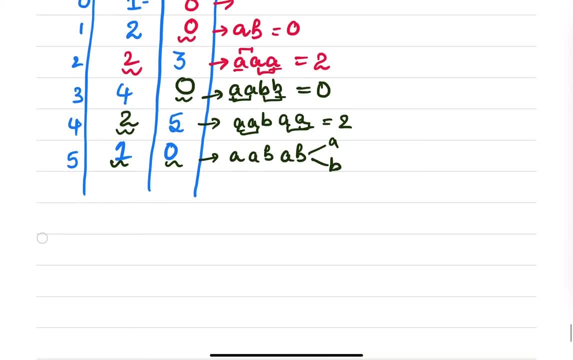 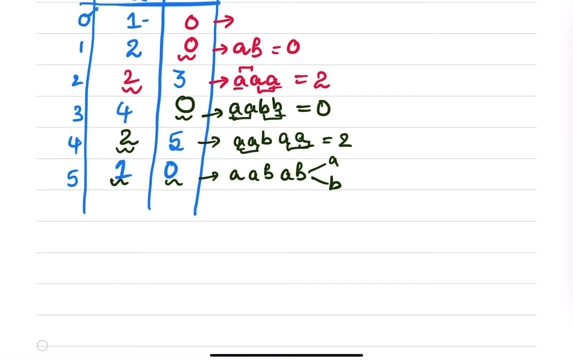 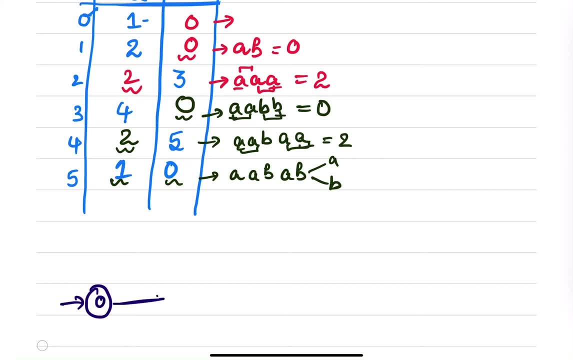 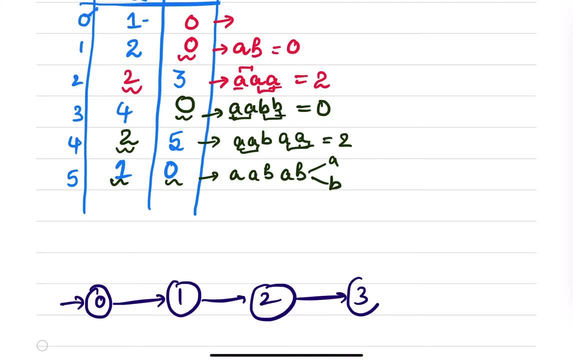 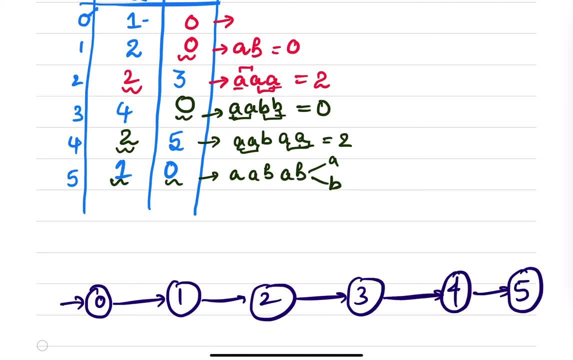 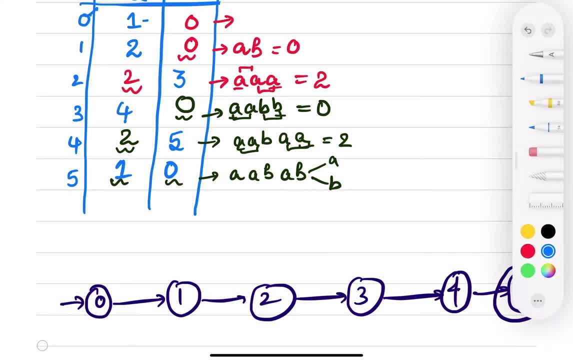 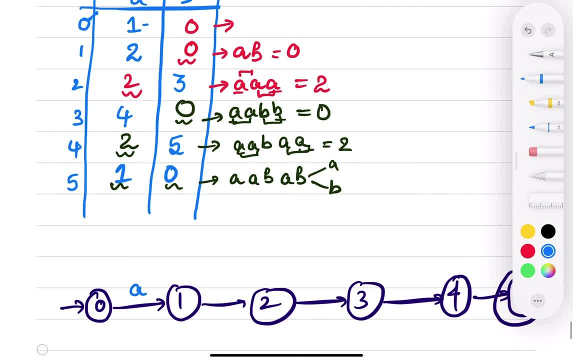 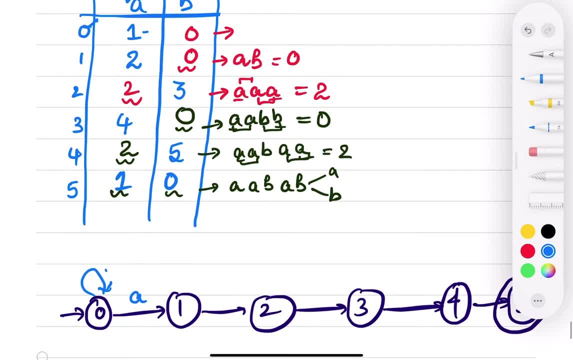 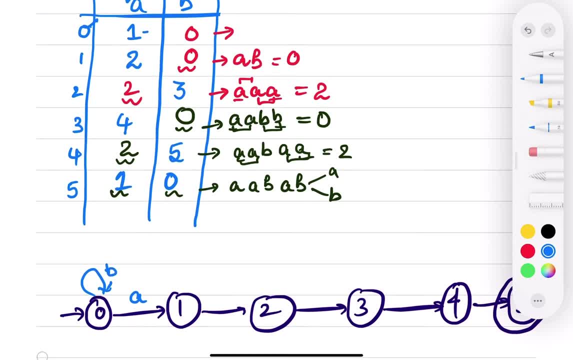 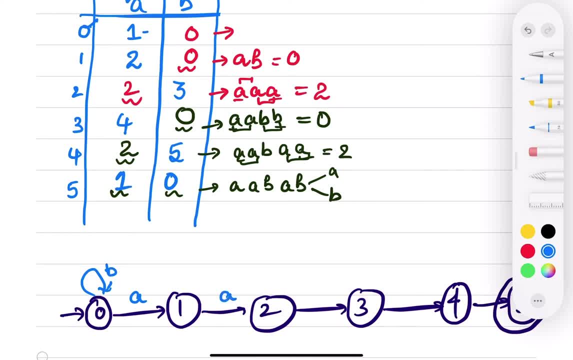 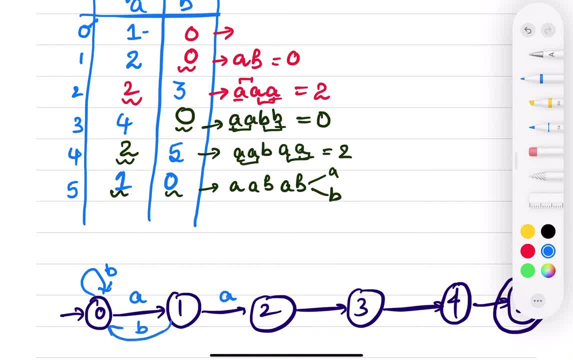 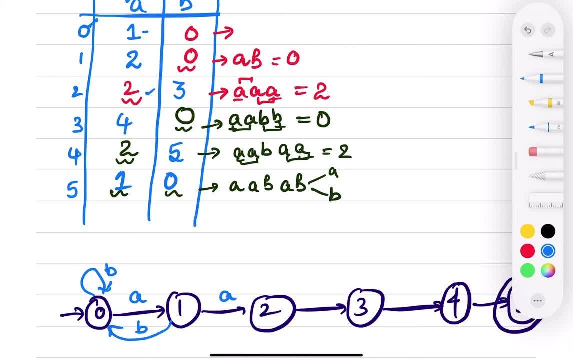 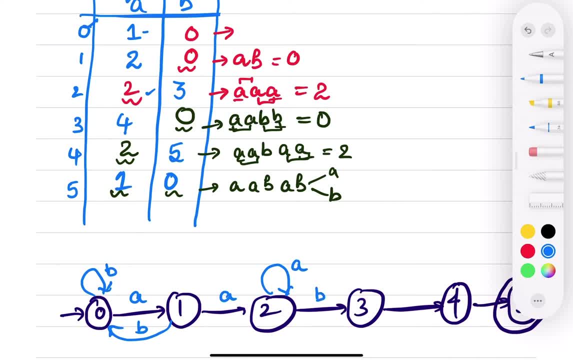 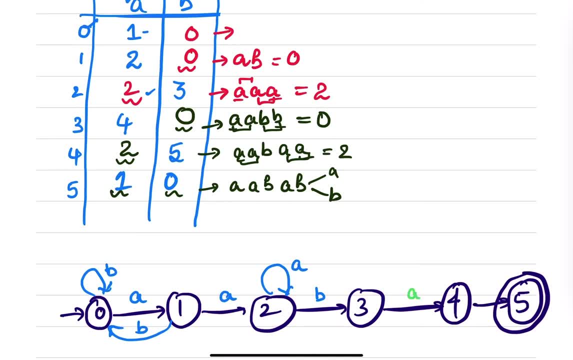 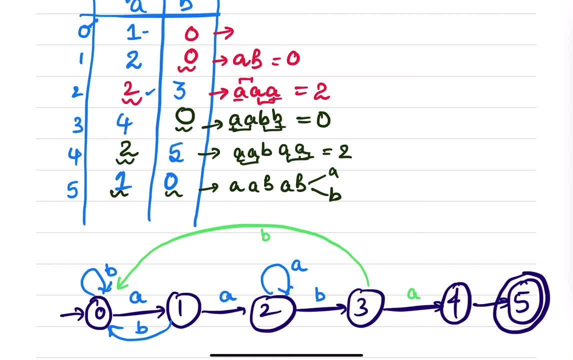 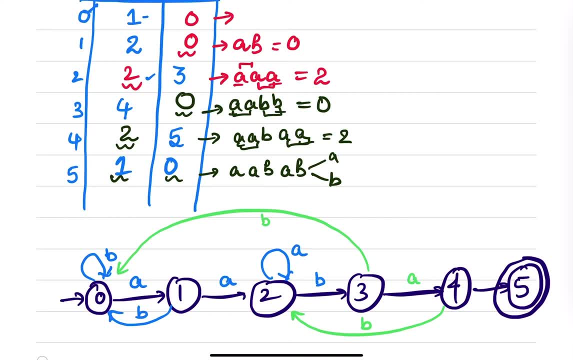 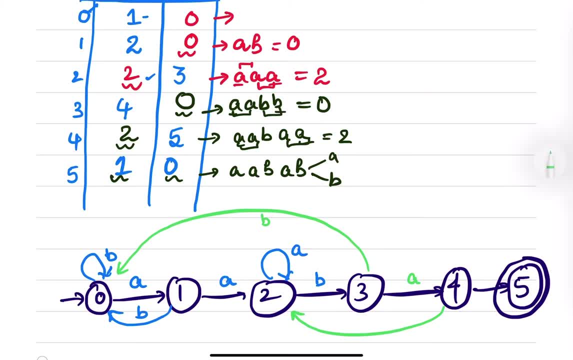 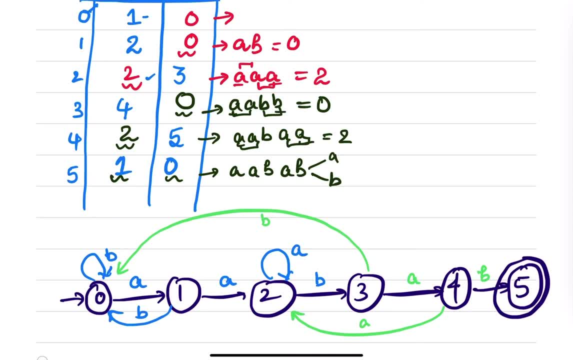 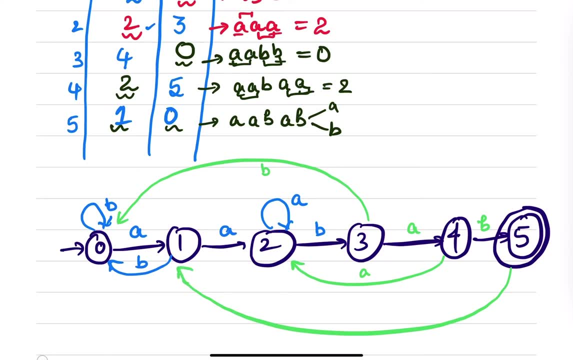 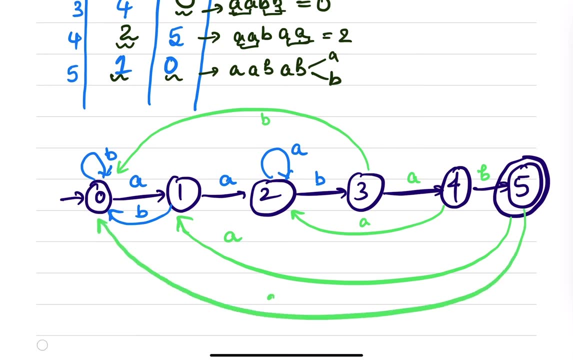 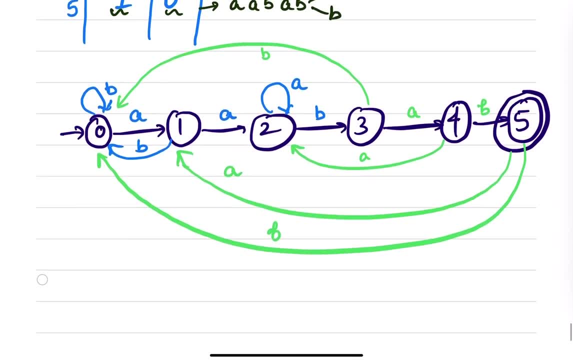 so this is your automata. now you have to traverse the string or you have to put give an input as your string. so your text string was a a a b a b, a a b, a a b a b a a b. so let's trace this so. 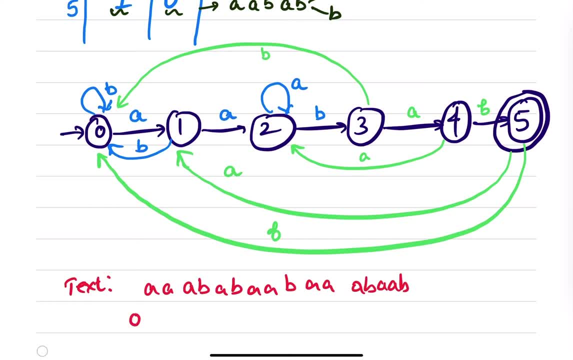 we will start with the 0 right, then you will take a, you will go to 1, then you will again take 2, a you will go to 2, then again a. you will again be in 2, then b you will reach to 3, then a you will reach to 4, then b you will reach. 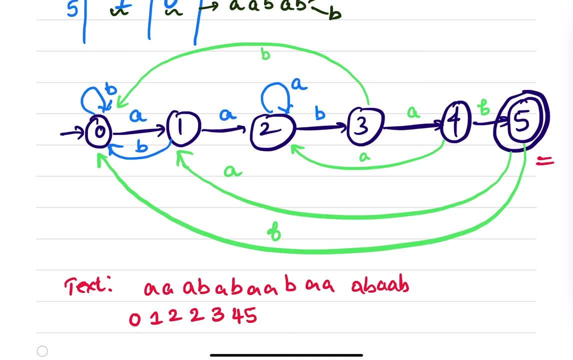 to 5.. see, you have reached to a final state here, so you can say that you already have travels, or you can say a pattern is found in a text, because you have reached to a final position. but for timing i'm just writing the complete execution, so you: 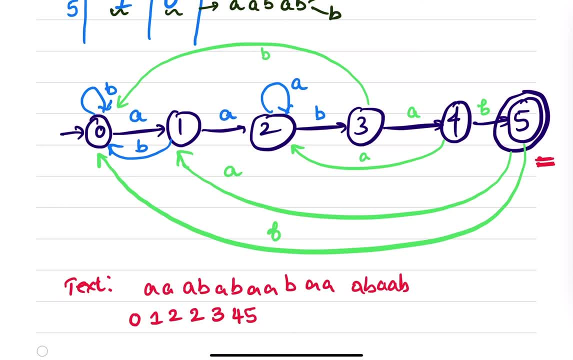 have. otherwise you have already got it right. you are here now. 5 is the final state, and you are already at the final state means this pattern is there in a string and you can see this: a, a, b, a, b was the pattern, right, but i'm traversing the complete text for you. so we were at five then.